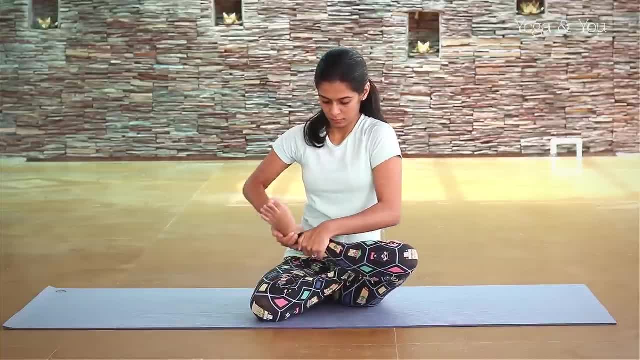 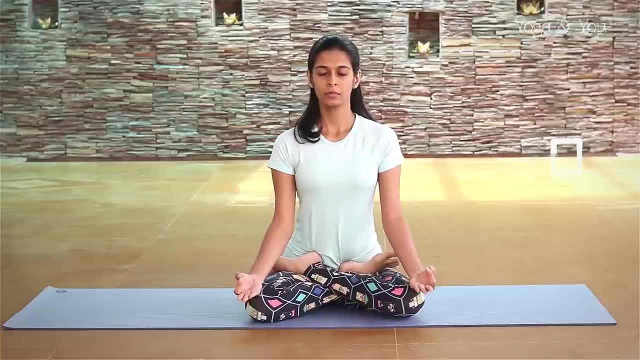 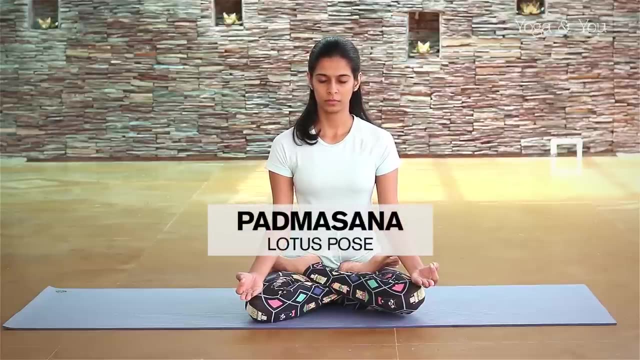 leg, bringing the left heel towards the right pelvic bone. Allow the knees to drop towards the mat. place the palms on the knees in Chin Mudra, with the thumb and index finger in contact. the eyes softly closed, Sit in Padmasana for a few moments, observing your breath and your spine. 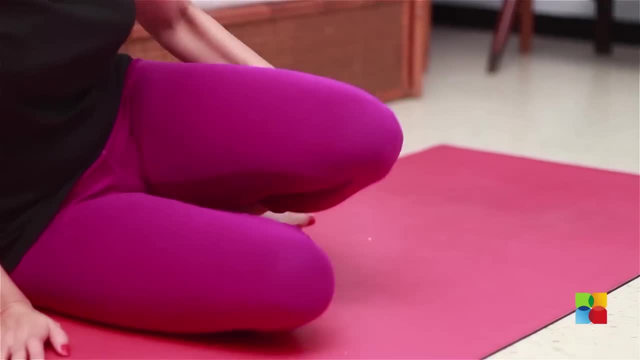 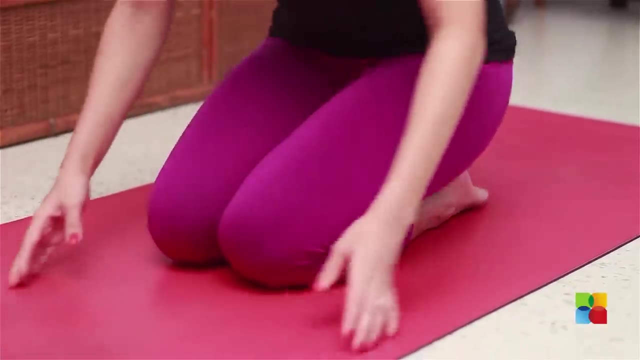 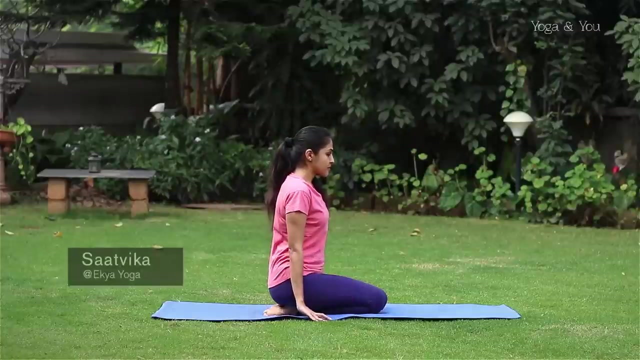 For Vajrasana, you sit on your heels or, if I have to show you, you sit on your heels like this: your toes flat, your palms either facing up or down. Sit in Vajrasana From here. lift your hips up and sit to the left. Take your right foot. 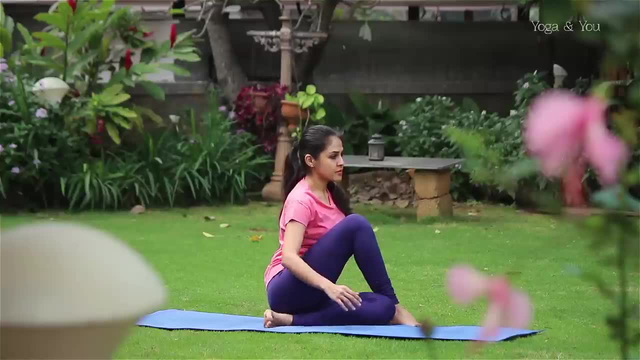 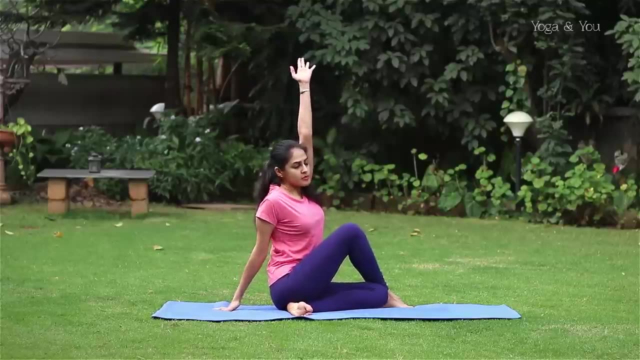 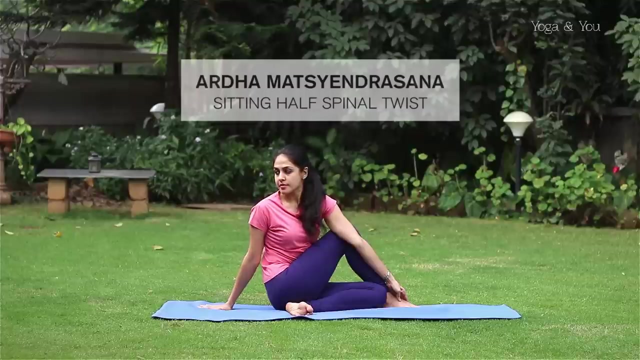 across your left knee and place it on the mat. Make sure your hip does not lift off the mat. Place your right hand behind you for support. Inhale, lift the left arm, twist and place your hand on the foot. Look over your right shoulder. 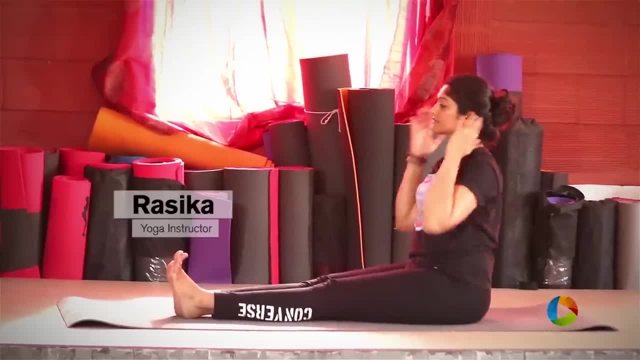 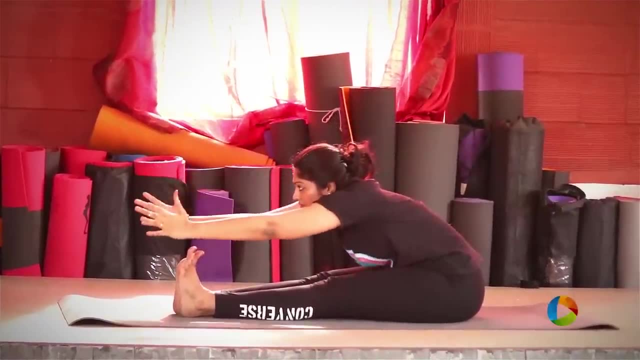 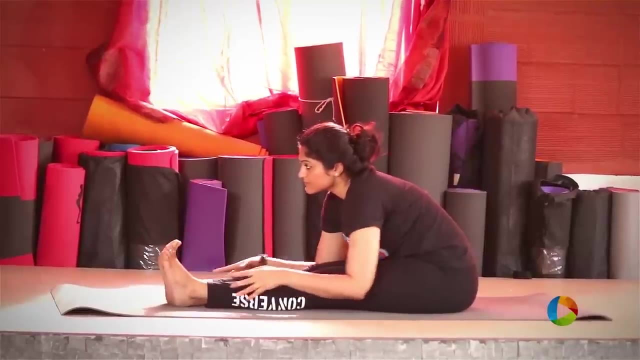 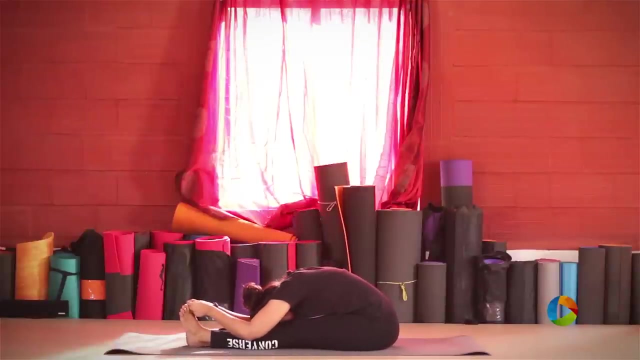 Good, Now you can do a full forward fold So you can catch hold of your toes, if you can reach your toes, or you can hold your ankles, calf muscles, wherever you are comfortable And pull yourself forward. So the aim must be to reach the front of the leg and not to reach 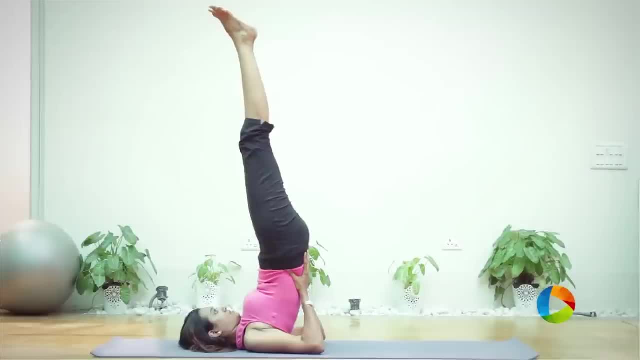 the forehead to the knee And from Sivangasana moving on to Halasana. you need a lot of core strength here. So just take your time, keep yourself comfortable and, without bending your legs here, inhale deeply and as you exhale, just push your hips down and bring your legs all the way up above. 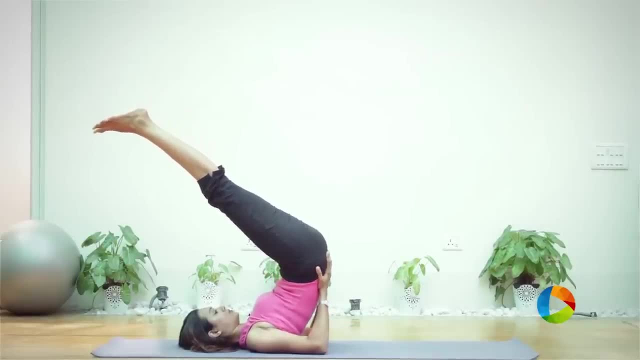 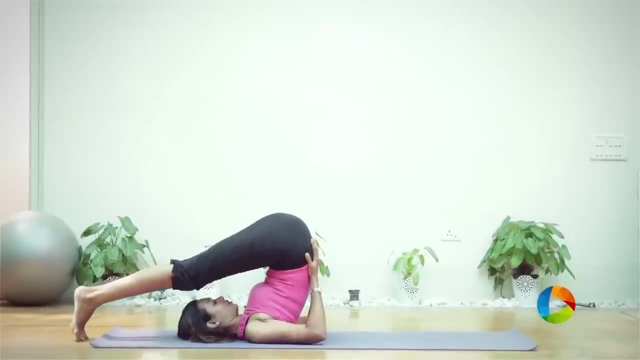 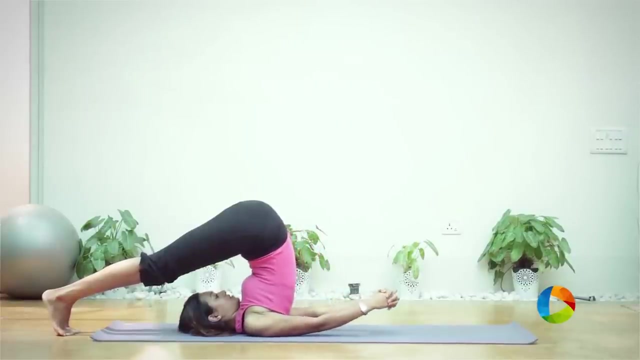 your head. So take your time, Do not rush into the posture. Keep exhaling, Use your core, Engage your core muscles and bring your leg all the way over your head. And now your hands can get interlocked here and bring it all the way down, strengthening.